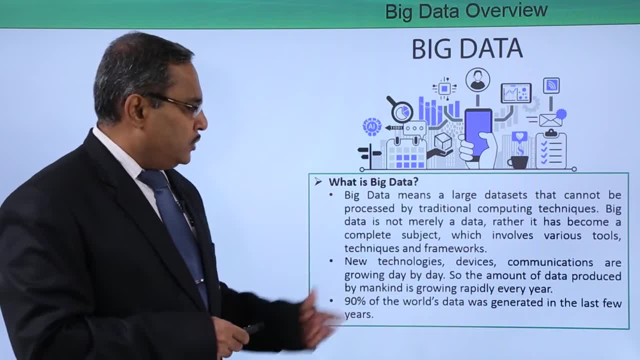 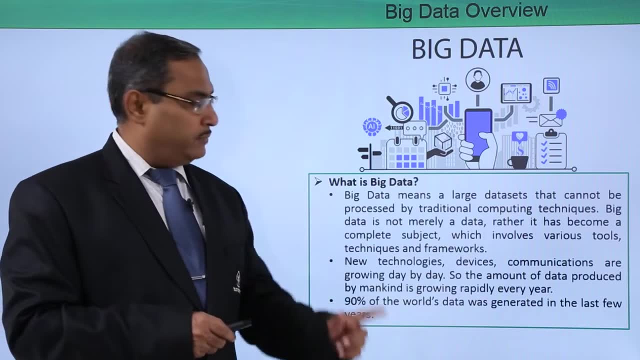 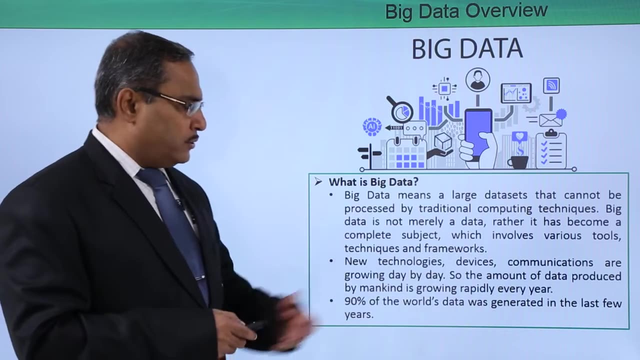 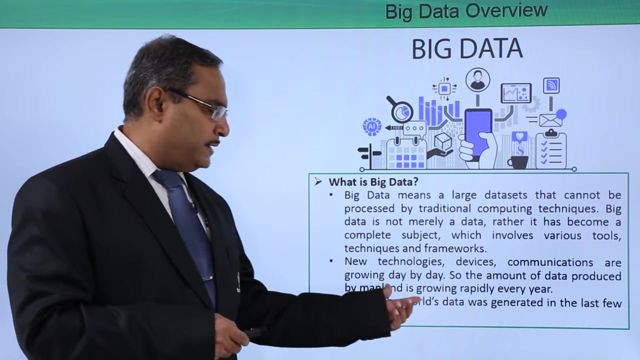 traditional computing techniques and systems. so big data is not merely a data. rather, it has become a complete subject towards the solution of the big data, which involves various tools and techniques and new type of frameworks, new technologies, devices. communications are growing day by day, so the amount of data produced by mankind is growing rapidly with the 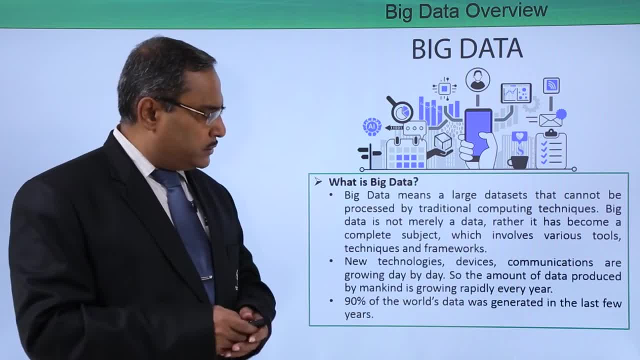 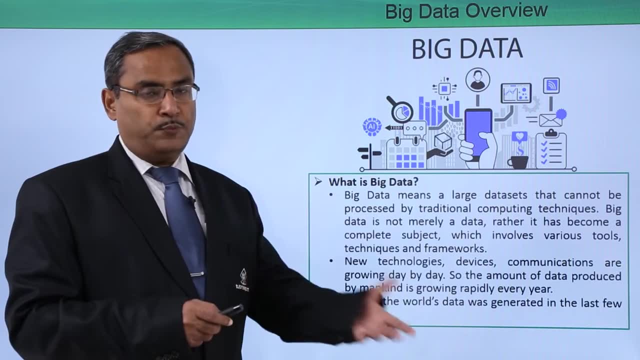 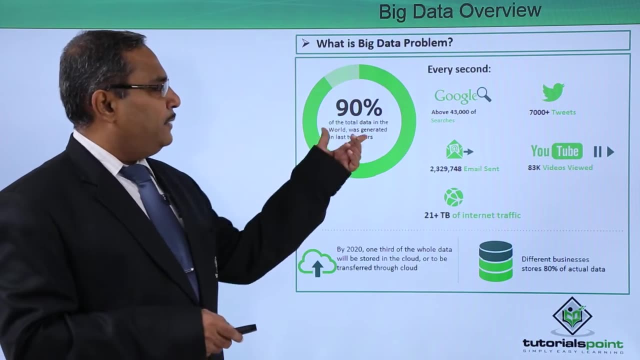 progress of the years. 90% of the world's data was generated in the last few years, so it is very alarming. ninety percent of the world's data have got produced in the last few years. let us go forward with some statistics. so just consider this one: 90% of the 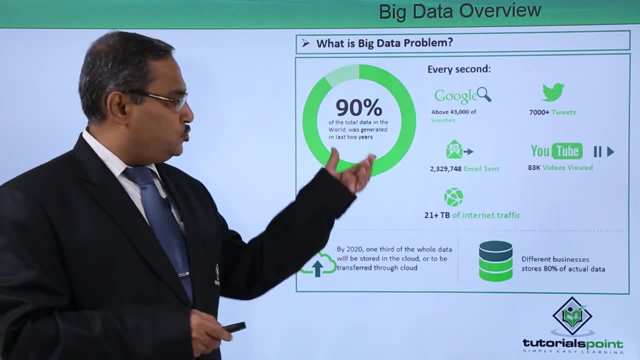 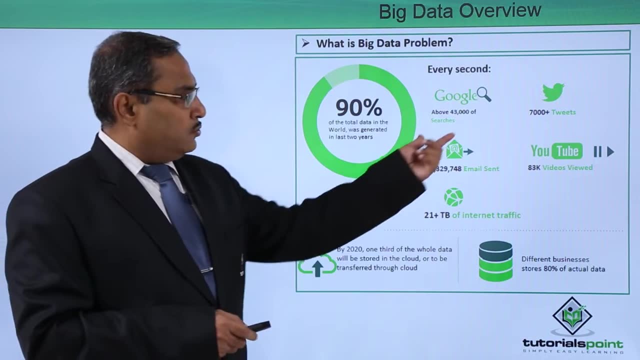 world data in the world of development or modernization are or at some cities in the developing world. world has generated in the last two years, last couple of years, 90% of the data it has got generated. so now for every second, Google is having 43,000 of. 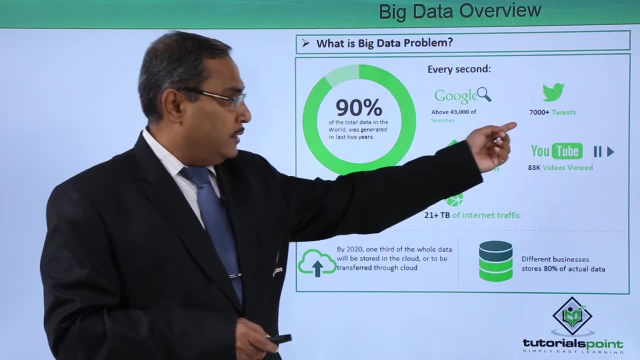 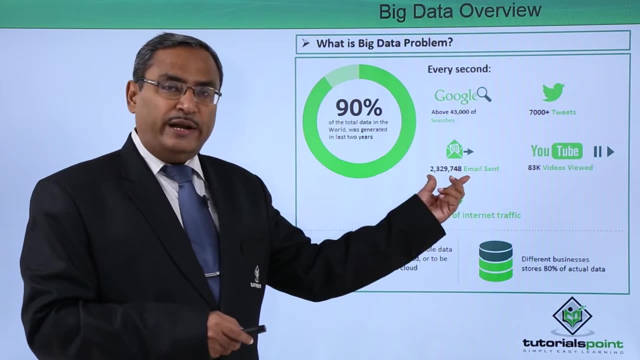 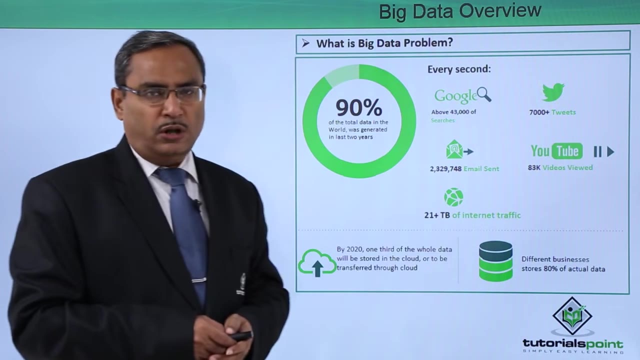 searches. just consider these figures per second. and here we are having 7,000 plus tweets on the Twitter per second. we're having almost 24 lakhs of emails are getting sent per second. we're having 80k videos viewed on the YouTube. we're 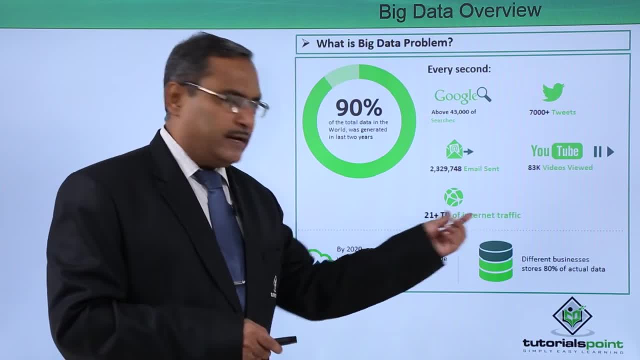 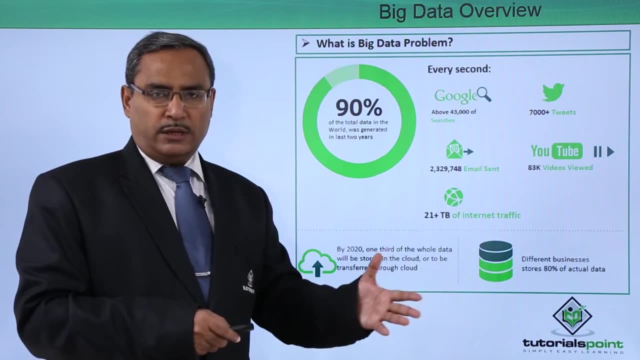 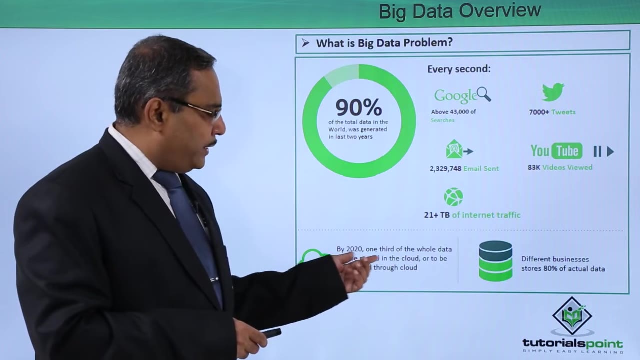 having 21 plus TB of internet traffic per second. so just see the volume per second we are considering here and if you go for the years, if you go to calculation for the months, it that would be a enormous figure. and by 220, one third of the whole data will be stored in the cloud or to be transferred to. 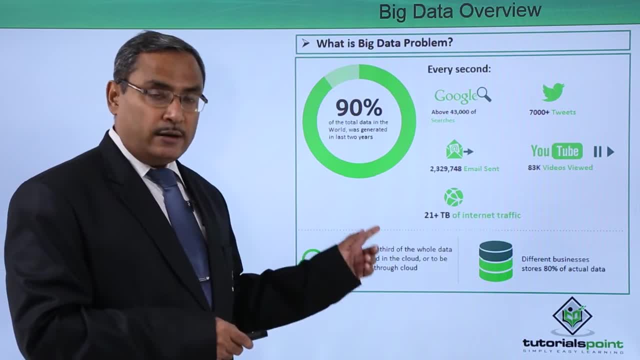 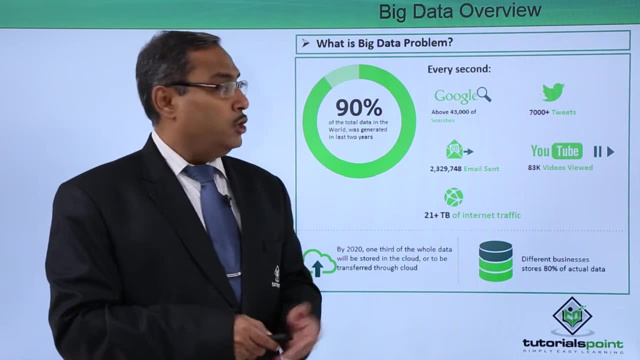 the cloud. so that's why it is also very much alarming figure and we are having that 80% of the business actual data will be stored on the cloud. so that's why big data has become a problem, has become a subject and we require some solution. 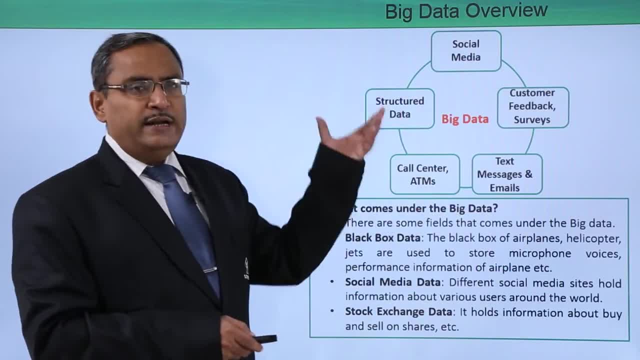 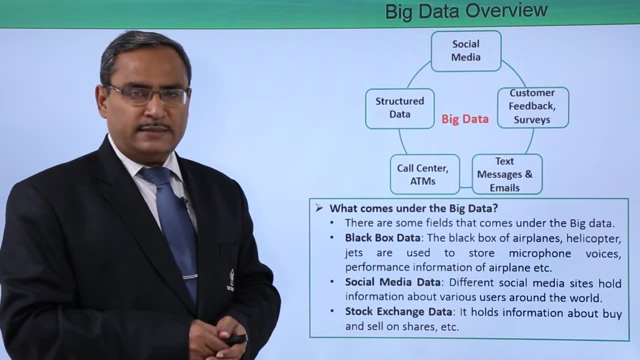 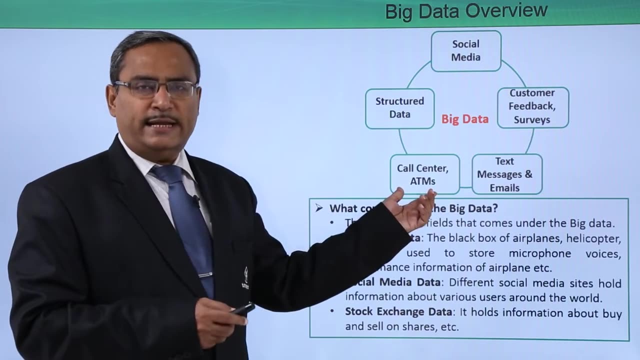 for that. so here you see, we're having different sources from where this big data is getting originated. we're having the social media, we're having the customer feedbacks and surveys, we're having the text messages and emails- and we we always do this one- and then call centers from ATM. so we're having so much.